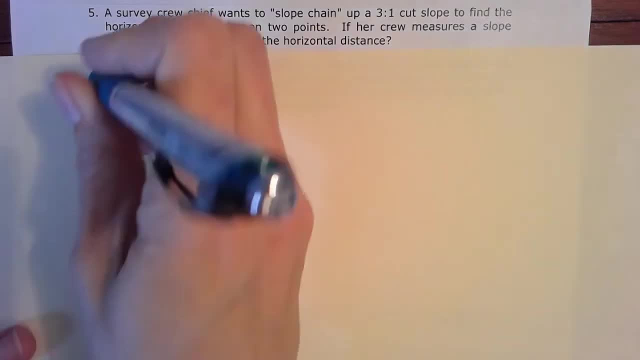 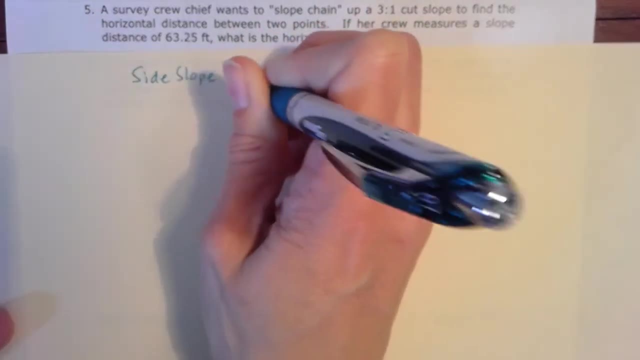 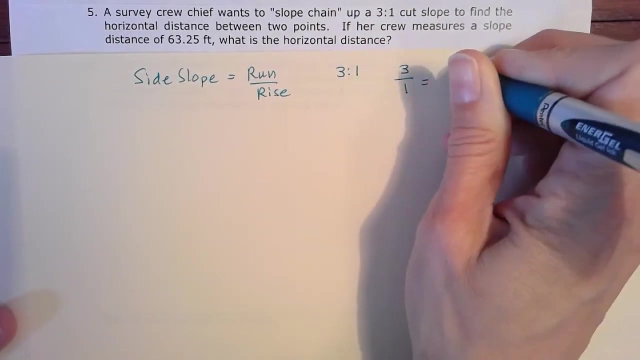 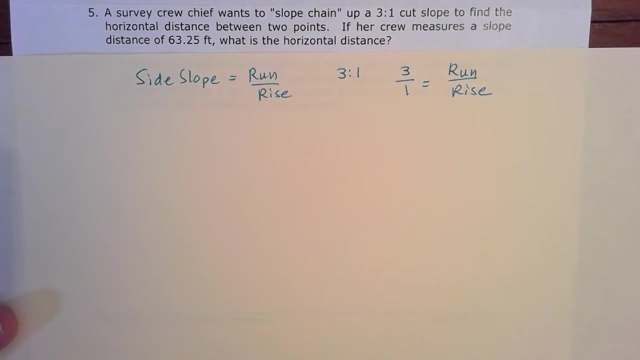 So we can tell by the way that this is written that this is a side slope, And remember that a side slope means run over rise. So we're told that the side slope is three to one. So we can rewrite that as three over one is going to equal some run over some rise. So we've got that base equation to start with. Now, in this case, we're given the slope distance, So we're actually given the distance along the angle. 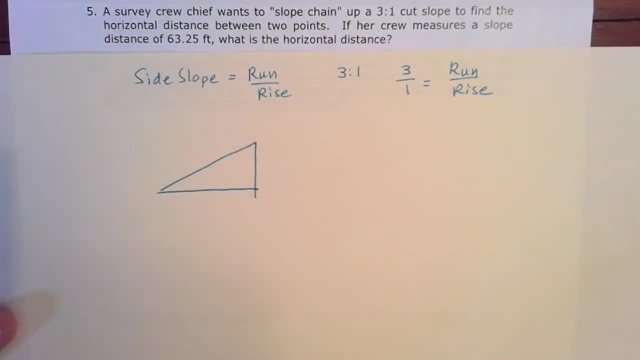 So that's what that means: to kind of slope chain up that, up that angle, And so we have the slope distance of 63.25 feet. So we're not being told an X, a run or a rise in this case, But we are able to figure out some information from this angle. So one thing we can think about is that this is the triangle. 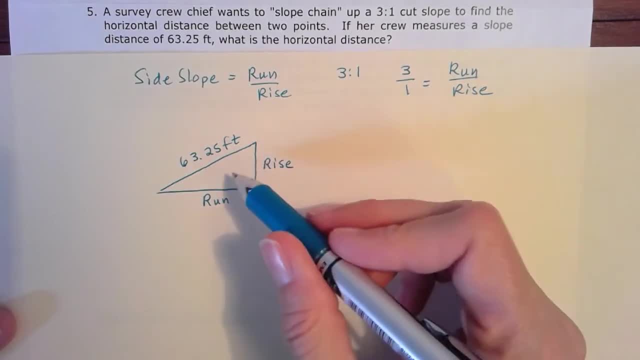 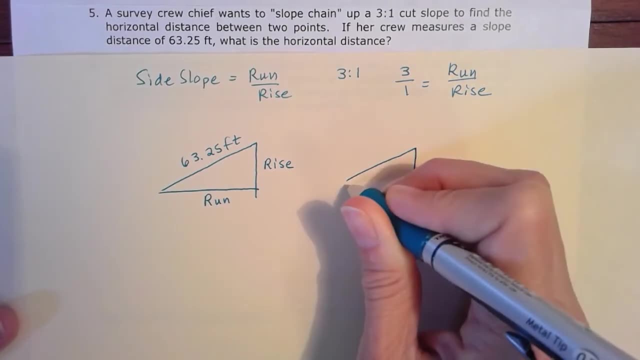 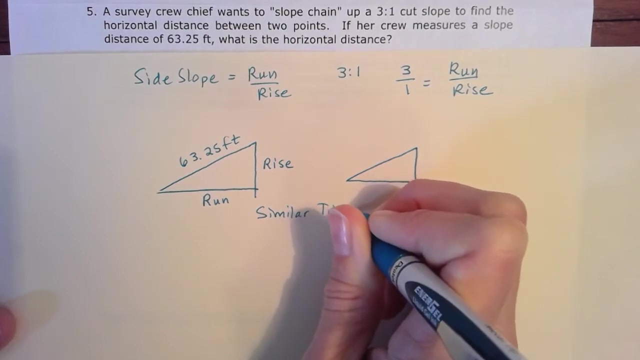 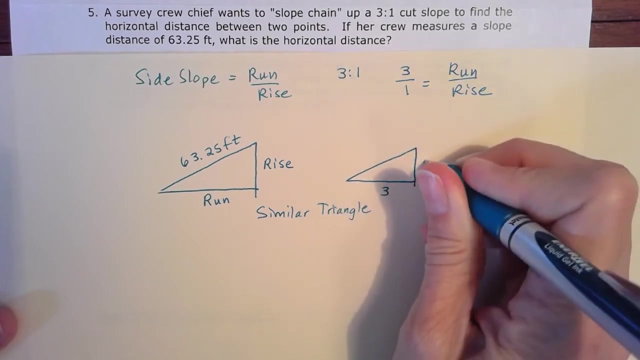 This is the triangle that is of interest. But we know that this slope follows this three to one pattern. So if we drew that triangle just kind of a base similar triangle, So we're going to look at these two similar triangles. We know that a three to one means that three is our run and one is our rise, So these two triangles are similar to each other. So we can know with these dimensions. 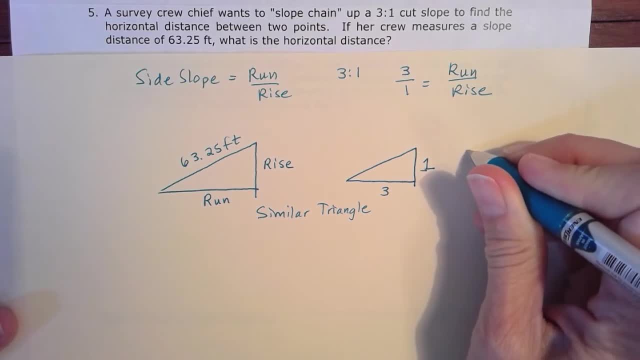 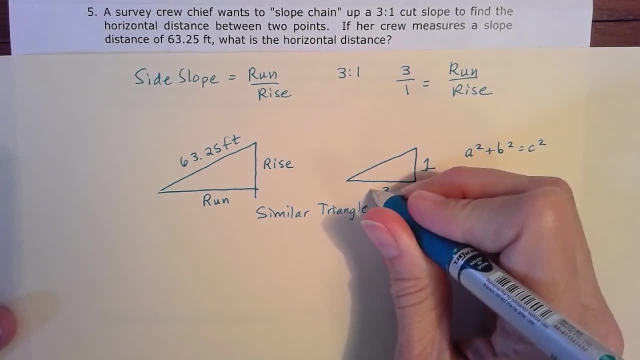 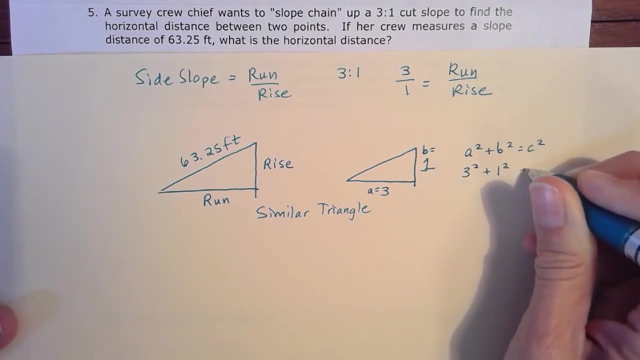 I'm using our Pythagorean theorem that, remember, a squared plus B squared equals C squared. Okay, if we call leg a three and leg B one, we wind up with three squared plus one squared equals some C squared here, So that becomes nine plus one equals C squared. So C squared is going to equal 10.. So C is going to be the square root of 10.. 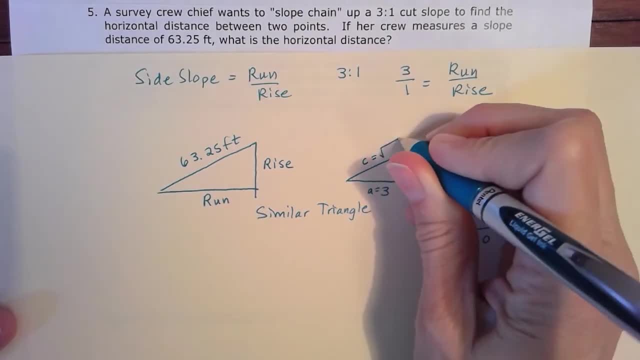 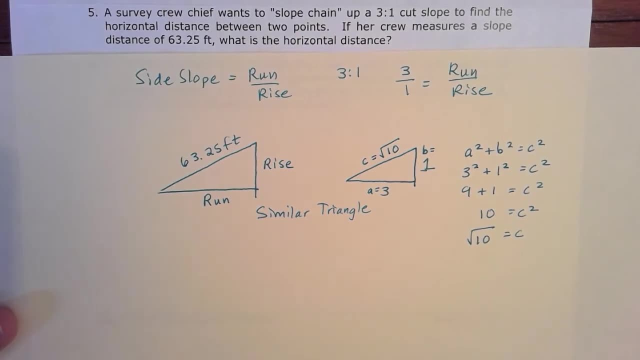 So we'll call that this leg C, our hypotenuse, and we'll know that that's the square root of 10. so now we have two similar triangles that we can write down relationships about. so we can say that on one leg the run is this unknown and we'll just call this X, since 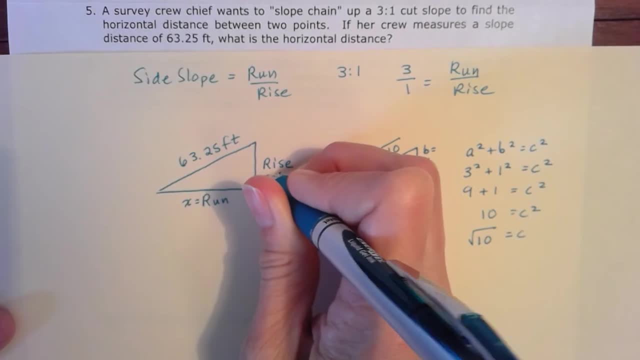 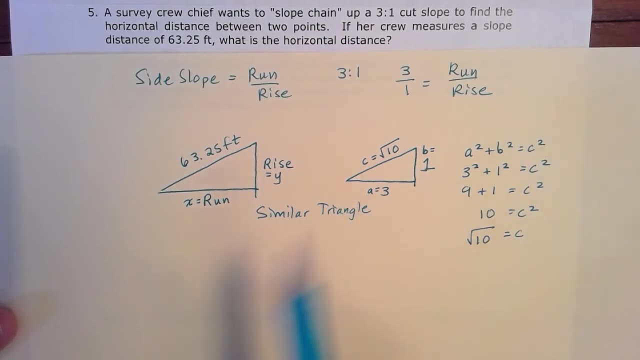 it's in the X direction and this rise is unknown and we'll call that Y. so we can say, because of similar triangles, that X is similar to this three leg, so I'll put three over X and then one is similar to this Y leg, one over Y, and then we can. 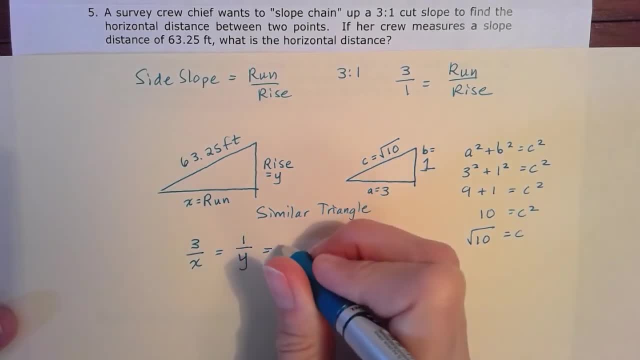 equate this hypotenuse square root of 10 to our sixty three point two, five and, if remember, in FEP statics when we have these similar triangles, we can pick any two of these relationships to set to equal to each other to solve for the. 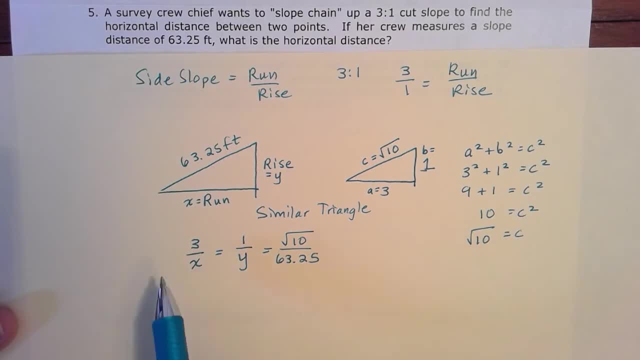 variable. we do have two variables here, so we got to get rid of one of these triangles and then we can write down the relationship between the two of these two equations. really, all we're interested in is the horizontal distance, which is the run. so we don't really care about the rise. so we can. 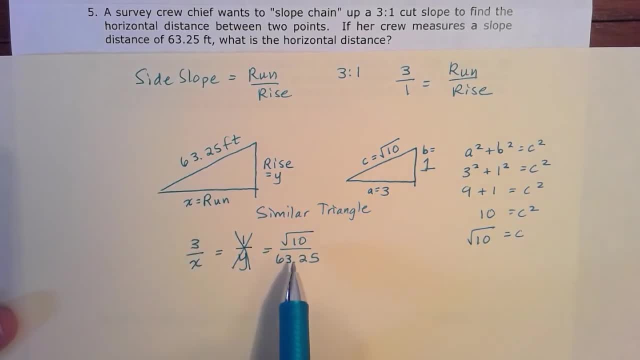 just cross that guy off and use these two equations and set them equal to each other. so let's rewrite them down here. so three over X is equal to the square root of 10 over sixty. three point two, five. I'm just going to go ahead and. 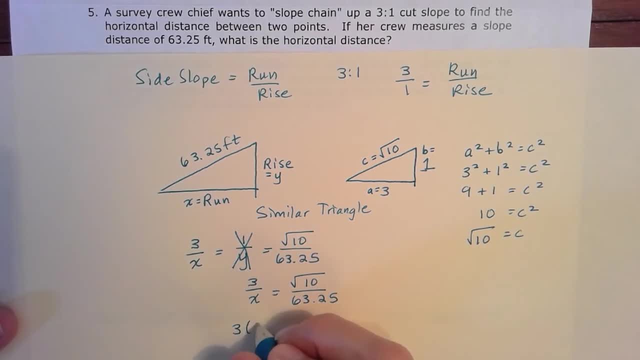 cross. multiply those so I get three times six. sixty three point two five is equal to X. and then we have the horizontal distance, which is the horizontal distance which is equal to X times the square root of 10, and if I multiply that out three times sixty, three point two five is going to give me. 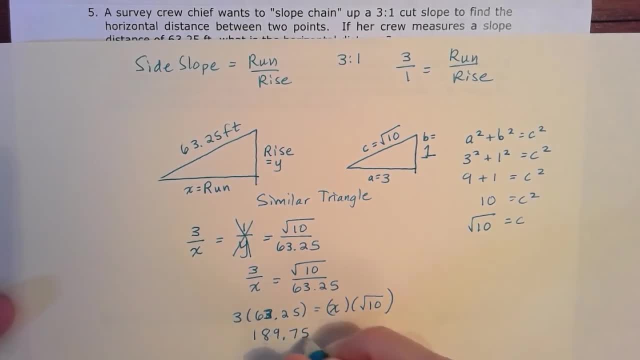 one, eighty nine point seven five is going to be equal to X times the square root of 10, but we'll just divide that square root of 10 by both sides, all right, so we'll wind up with that. and then, if we put that into our calculator, 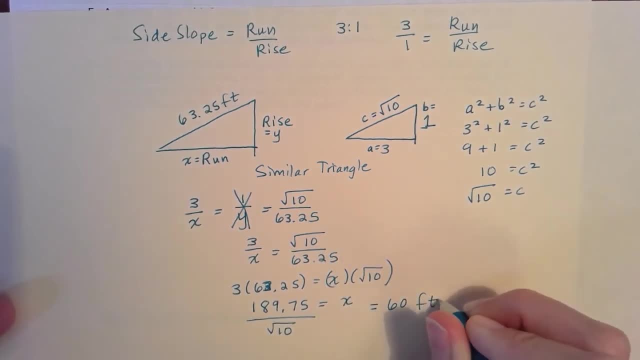 we do find that X is equal to 60 feet. all right, so that's going to be the hard horizontal distance of that three to one slope side slope, when we know that the slope angle is equal to sixty three point two, five feet.